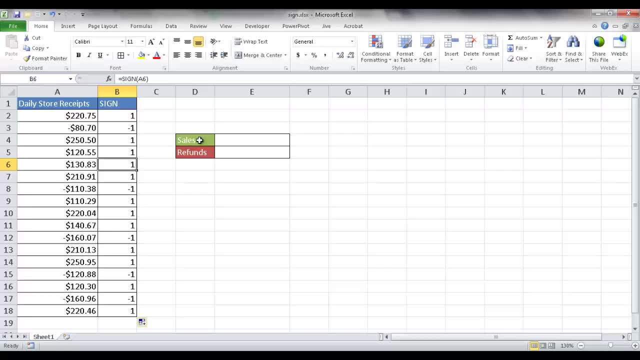 So what can we do with this number? Basically, if we wanted to differentiate between the sales and refunds, we can put it into another formula. So I want to be able to sum up all the numbers that are positive and all the numbers that are negative. 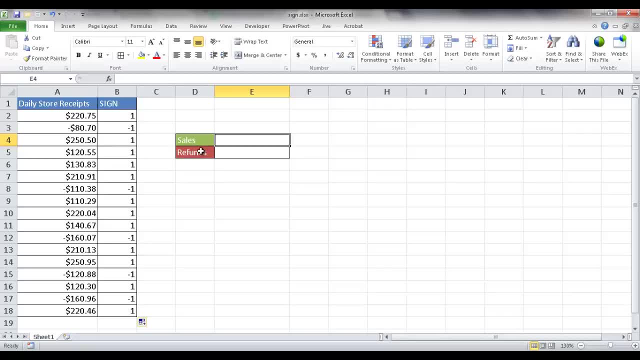 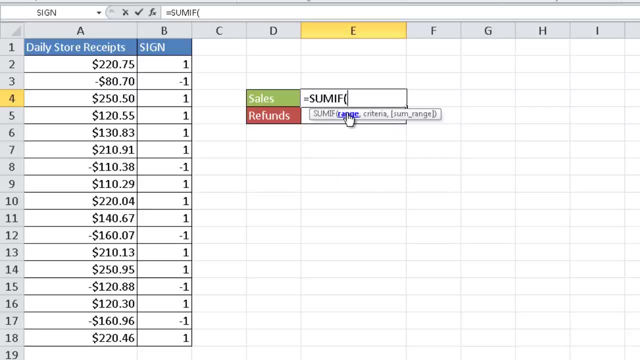 Meaning all the numbers that are positive are sales, all the numbers that are negative are refunds. So I can use the SUMIF function. So if I type SUM and select SUMIF here, what I can do is select my range. So this is the range where I want to match it up to my. 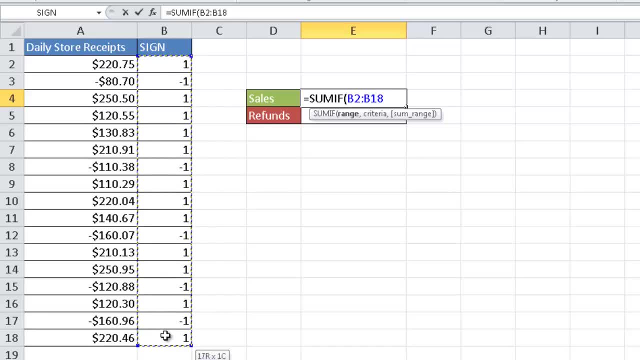 criteria, So this range of the ones and negative ones, and my criteria is for the sales. I want to indicate a positive one, So just the one here, And if it matches that particular criteria, I want to sum up those adjoining cells which match up. 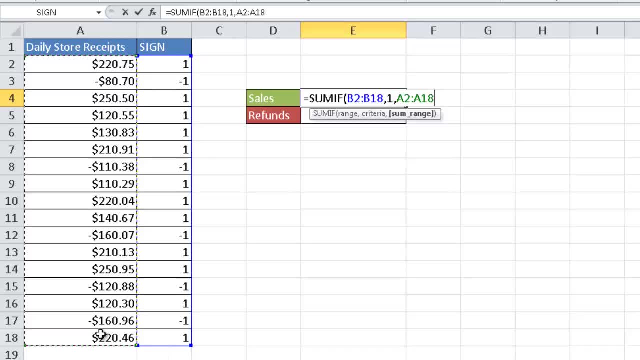 So I'm going to select this range from A2 to A18 and press ENTER. So what it's done is it has looked at this criteria, find out all the cells that have a positive one and summed up all the adjoining cells here And I can do the. 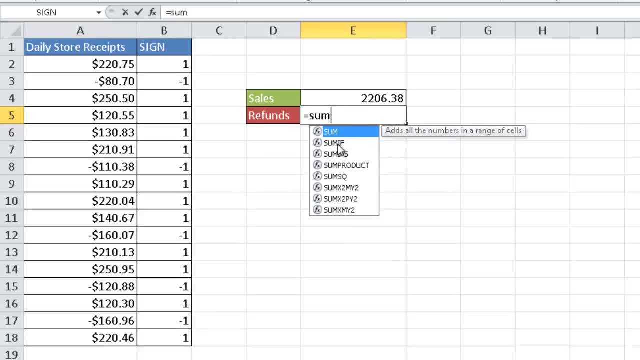 same for refunds. If I type equal, SUMIF, I'm going to go and double click that and SUMIF, Select my range here and type a comma, negative one, and then what's my sum range? that's over here, And then go ahead and press ENTER. It'll give me minus. 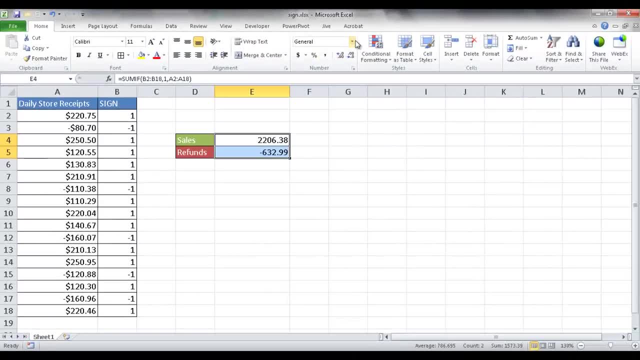 $632.99.. So I can just go ahead and format that now to currency to make it look nicer. So you can see our sales here are a little over $2,200, and our refunds are a little over $600.. And just to verify this, since the refunds are a 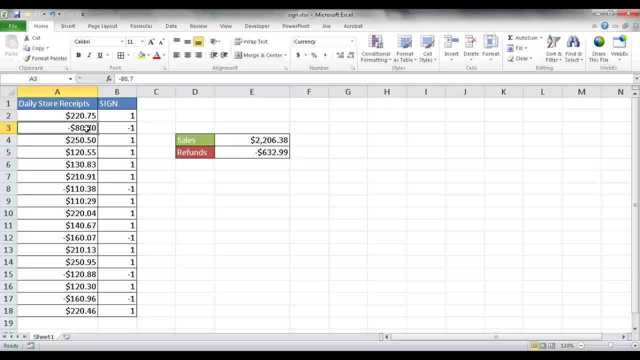 little bit smaller. I can verify that by clicking this, pressing the control key, clicking on here. that's the other negative one, that's the other negative one, that's the other negative one and that's the last negative one here. So if I look down here, it's summed it up to negative $632.99,. 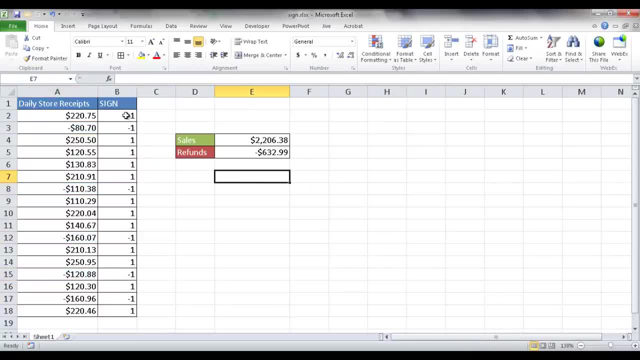 which is my value here. So that's one of the ways that we can use the sine function. In and of itself, the sine function doesn't really provide you much capability, but when you use it with other functions, you can see that there's. 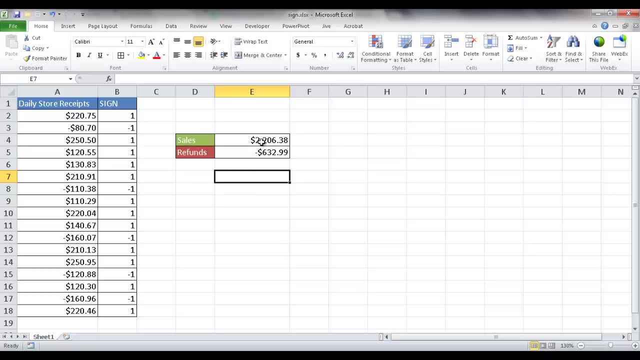 actually a pretty useful purpose for it, So I hope this helps. Thanks for watching. I hope this helps. Thanks for watching.